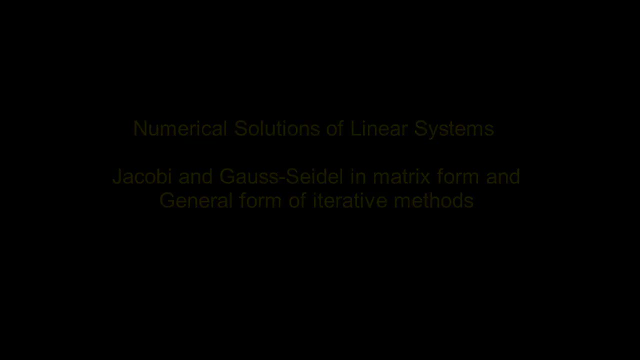 So now, in order to get to the next step, which is analyzing, doing some error analysis and specifically looking at the initial guess: whether you know guaranteed that any initial guess will actually work for the Jacobi or the Gauss-Seidel? we need to look at this. 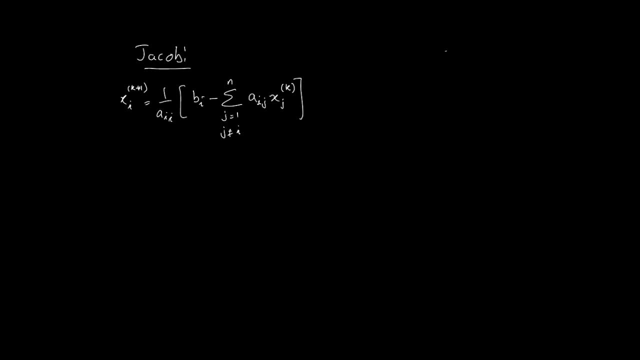 in a more matrix format so we can do some analysis on generalized iterative methods. In order to do that, we have to first write Jacobi as a in matrix format. essentially. So, if you think about it, what that means is the left-hand side. we can easily just 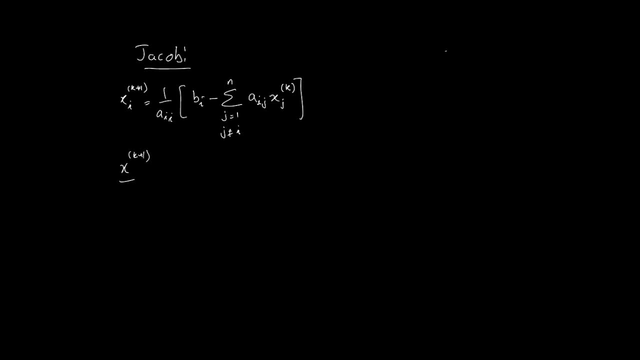 say xk plus 1, the vector okay, and that would mean that would entail all the x1, x2, x3 and so on. Now, if you take this piece here, this one here, let's identify this one. 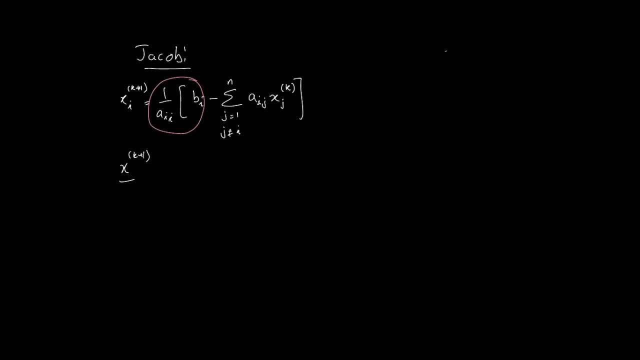 first. So that is basically what those values look like. are they're something like this? So they're b1 over a11,, okay, b2 over a22, and so on and so forth. So this is easily done by the following: We introduce the matrix D. okay, we introduce the matrix D, which. 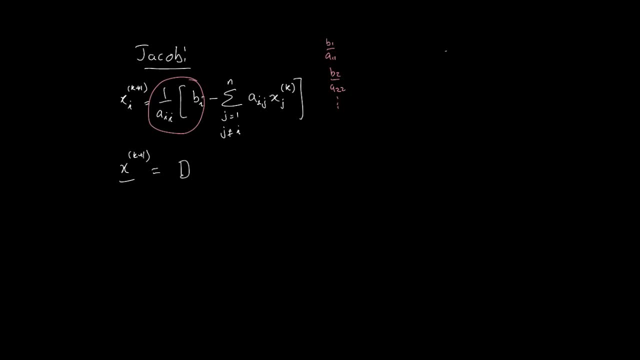 is in fact where D is in fact equal to is the diagonal matrix, which means D would be, for instance. in this case, D is just a1100.. So we have 0a22, you know, 0 all the way through, 0 all the way through, all the way. 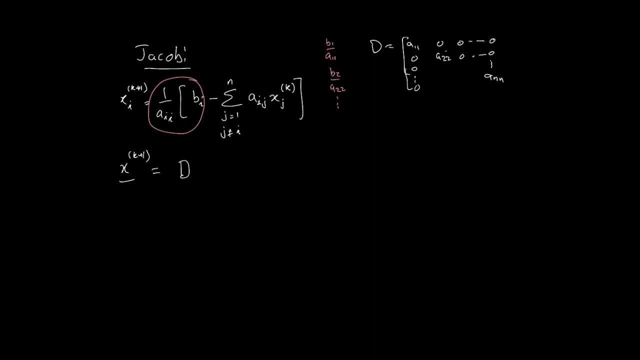 down to ann and you've got 0s all the way down here, 0s all the way down here. So anyway, it's this diagonal matrix. So D is this diagonal matrix. Now, you all know, you should know. 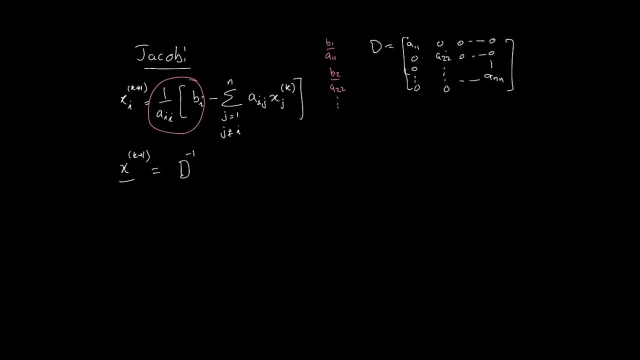 that D inverse, then, is simply 1 over a11, 1 over 8.. So D inverse is in fact, just 1 over a110 all the way through, 1 over a22, all the way down to 1 over ann, and there are 0s everywhere else. okay, So? 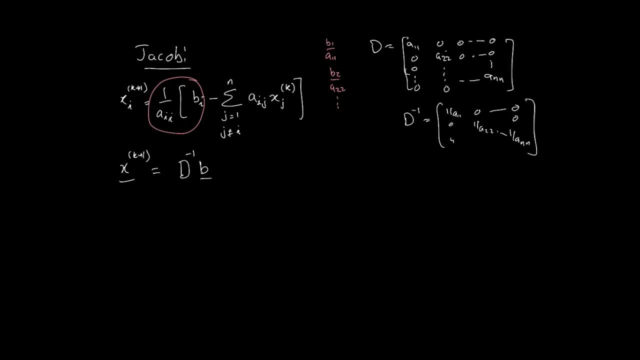 just a quick. so D inverse times. the vector B should take care of the should take care of this first bit. Then we'll say the following: Now, this is. this requires a bit more understanding. The next part is this- I'm going to write it down for you: I minus D inverse into the. 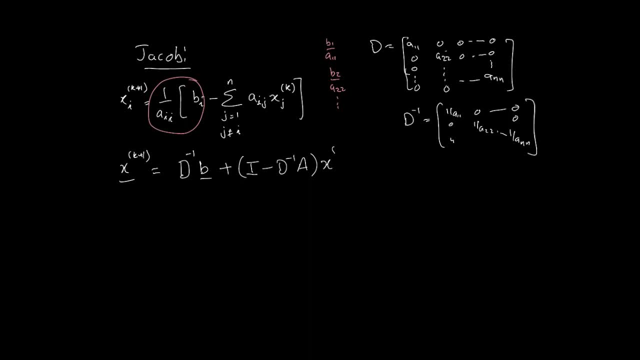 iteration, The coefficient matrix A times the vector K, in fact. Now, in order to motivate an understanding, I'm going to look at the 3 by 3 case, just to explain how this works. So hopefully you understand the first two. So what I'm going to do is I'm going to look at this bit. 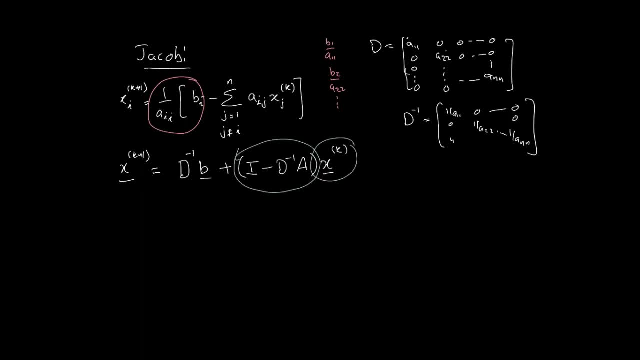 here how this works essentially, along with, of course, multiplication with this. So, in order for you to understand this, let me let's just ignore the XK and look at I minus D, inverse A for 3 by 3.. So for, for instance, when n is equal to 3, when n is. 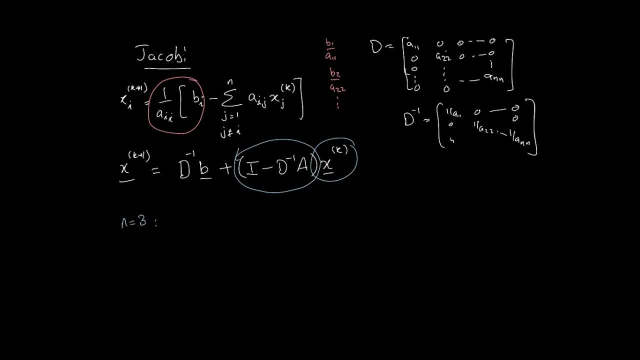 equal to 3,. our situation is something like this: We have, so we have something like this, So we have the, the identity matrix 3 by 3.. This is just for demonstrating demonstration purposes, And we have 1 over a11, 0, 0, 0, 1 over a22, 0, 0, 0, 1 over a33, and that is. 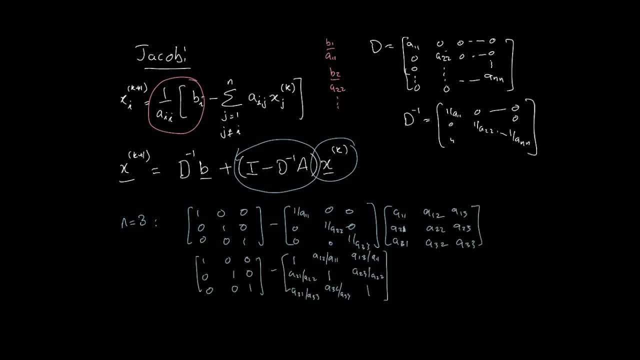 by a 1: 1. so we have this situation now. interesting that when we multiply these two together, so we get this. now you can see here- this is what's interesting. you see, these ones and these ones. when we subtract these two matrices we're going to end up with- in fact, this is going to become- all of these will disappear, and 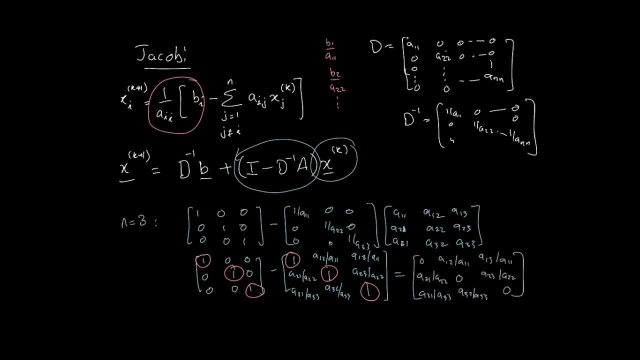 all that will be left is the following: so we end up with this matrix and now, hopefully, you can see that that, in fact, is is actually giving us this over here, so I hope that helps you to understand how this is, in fact, the Jacobi. so now, 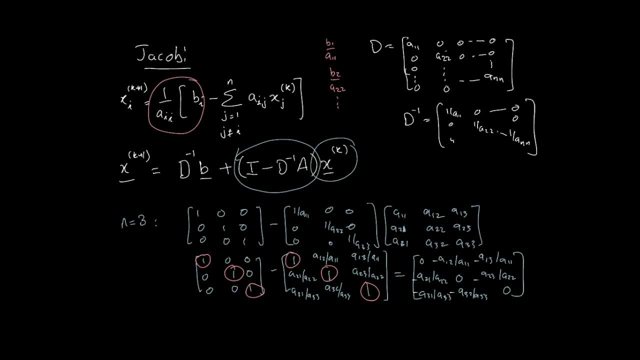 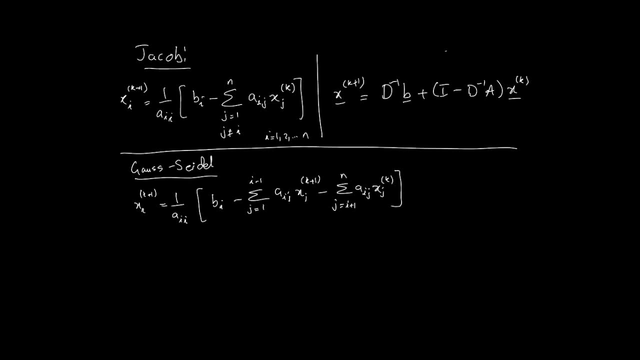 I'm gonna clean this up and we'll look at next the Gauss Seidel. okay, so now Gauss Seidel, bit more complicated. what I'm gonna do for the Gauss Seidel is: I'm gonna take the Gauss Seidel and I'm gonna take the Gauss Seidel and I'm gonna. 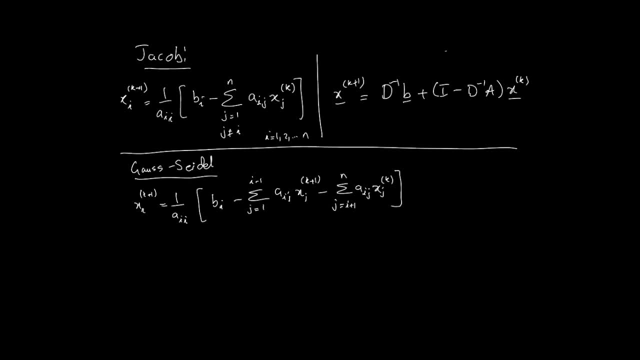 first is: I'm gonna take this AII across over here. I'm sorry, wait, sorry. so I'm gonna take this II across to here, so I get a II X, I K plus 1. so basically, what will happen is: I'll end up with: I'll end up with: I'll end up with this, if I have. 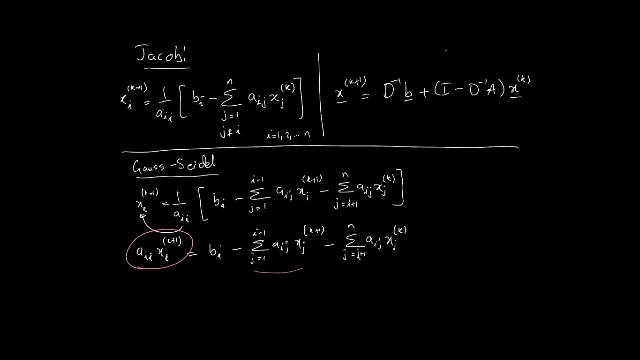 now look at this, look at this term here and look at this term here. of course, these can be added into each other, so if I bring this to the left-hand side, I'm gonna end up with, I'm gonna end up with just here. a summation from J equals 1, all the way up to I, in fact, okay, all the. 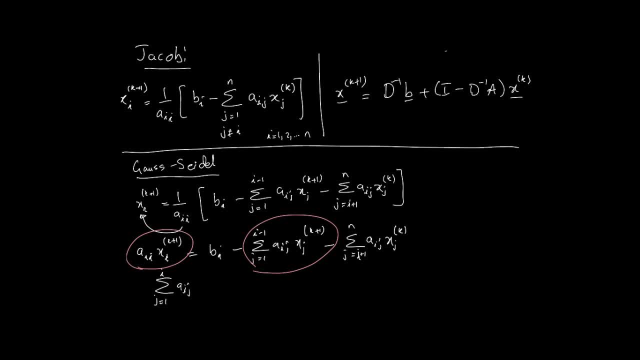 way up to I of AIJ. okay, because this is I minus 1 on this side, and then I have the I over here. so when I add these two, I'm gonna get everything up to I, in fact, and that's gonna leave me with the other side. with what will you see here? 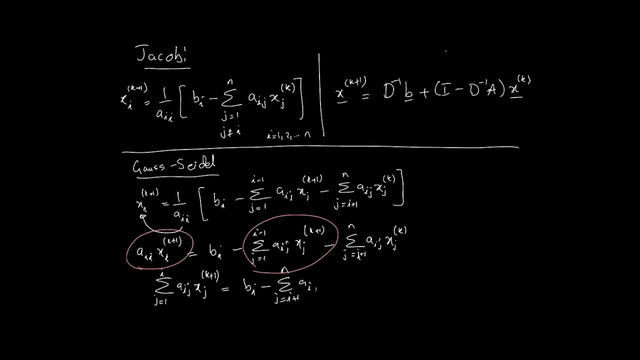 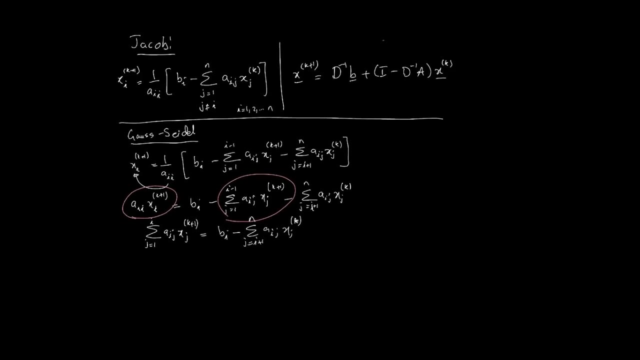 which is the I plus 1, all the way to N and the AIJ, X, JK. all right, that's the K, at it red. so that's just. that's just. I'm rewriting it now. if you look at this carefully, what you will notice, in fact, here, what's interesting, is that this: 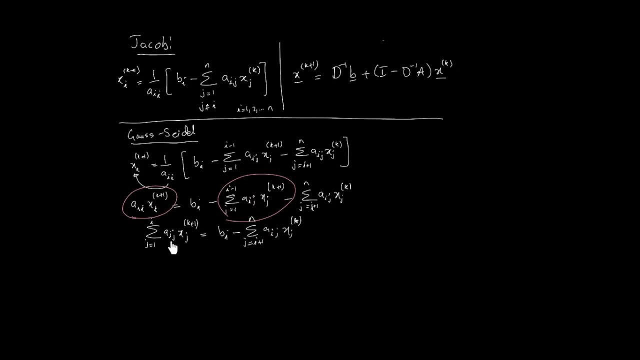 this over here is, in fact, what's gonna. what's happening is, as we count from 1 to I, we're essentially counting the lower triangular part of the triangle. in fact, these are all the lower triangle entries. so what we can easily do here is, if we define L on the side- I'm gonna do that here. so if I'm, if I say L is equal, 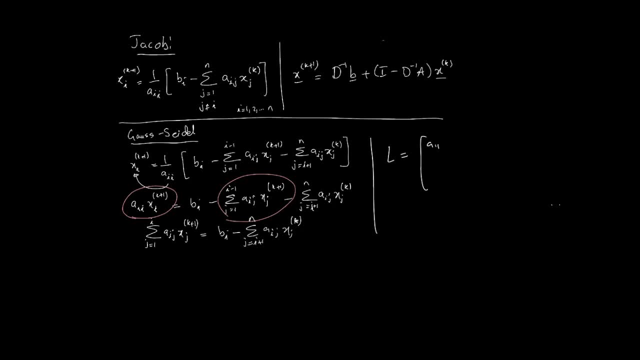 to the matrix, which is a, 1, 1, all zeros up here: a, 2, 1, a, 2, 2 zeros all the way down to a n, 1, a n, 2, a, n, n. so if I define this matrix, L, OK, which is not the same as the lower. 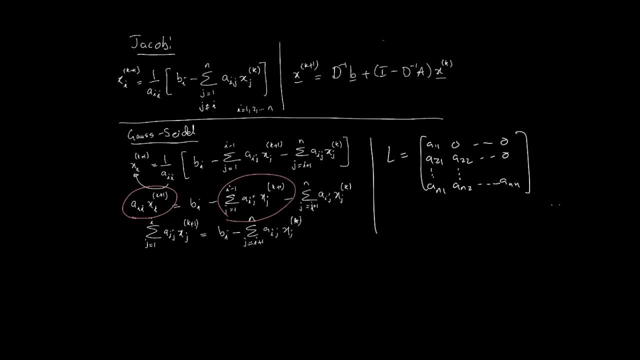 triangular matrix in LU decomposition. do not get confused with that. this is a lower triangular matrix which has these: just the lower triangle, basically, of a in that particular case. in this, the way I've defined it now, a is in fact equal to L plus you. OK, so the lower triangles part and the upper triangle of this matrix. ok, that's. 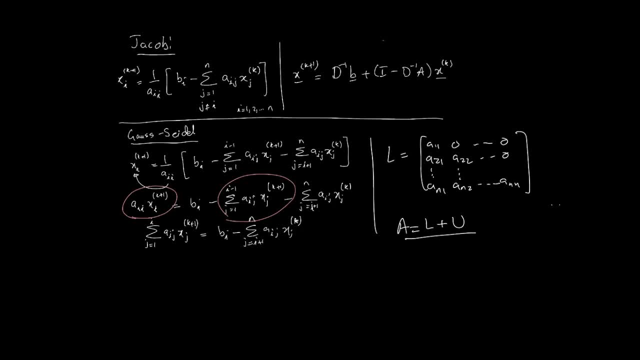 essentially the way I've defined it. Hierarchy: L, L And Tu, D, LIKE Z with A and D. this is one of the two right squares in the The upper triangle and the upper triangle on this matrix. ok, that's essentially the way we could define it with this l. just take it away from a the l, what you have here, in fact. 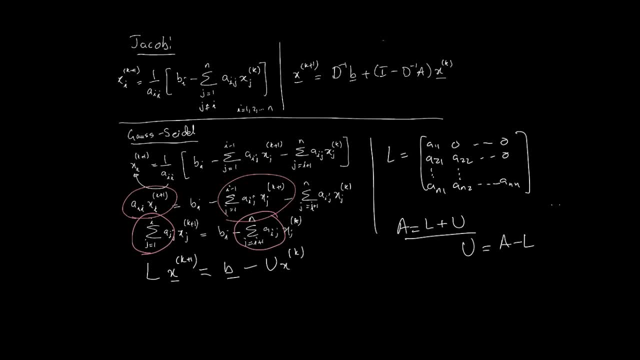 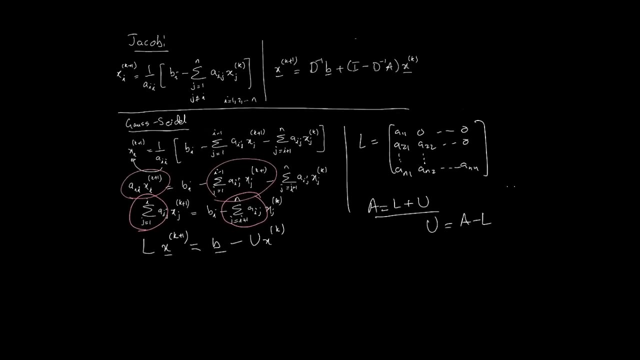 these coefficients are showing us what, when we take away the lower triangular part, the upper triangle remains. so that means we can write in matrix form as this: i hope you get that now, if we just play with that a little bit more, which is then: after that, it's quite straightforward. 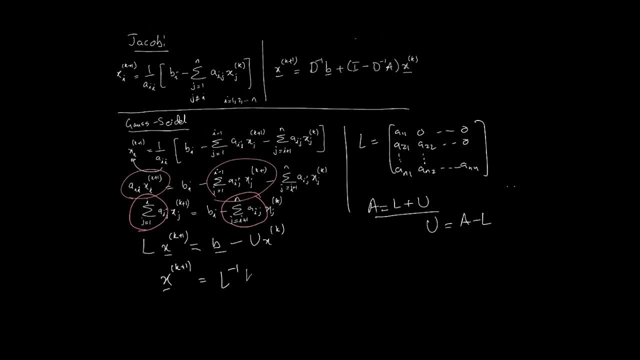 if we just rewrite that as l inverse b, okay, and minus l inverse u x k, so that is in vector form. now we can simplify that a bit further and then we'll do the following. just a little bit of matrix algebra, i'm sorry, will help us with this. if you notice, here the u, u is just a minus l, so 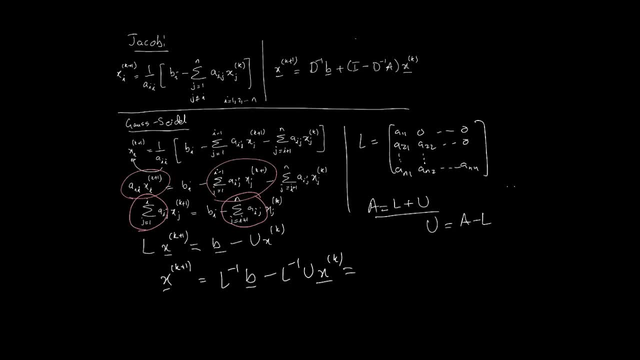 this means this is just equal to. this is just equal to, in fact, l inverse b minus l inverse into u, and u is in fact a minus l. so if i put that in here, there's my x- k, then this can be. it's just going to be equal to um l inverse b. 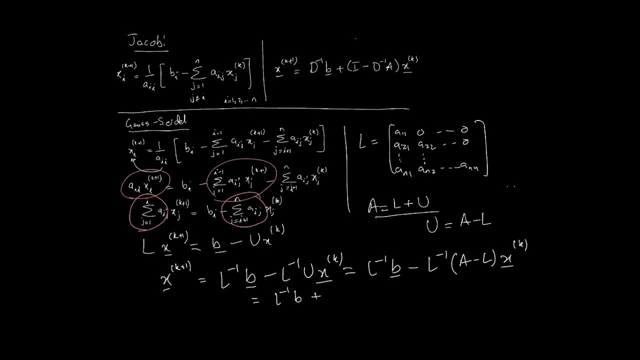 okay, plus, uh, i, because that goes in and essentially because of the well, in the matrix that comes l inverse l is just i, so that will become plus. i take it out and rearrange it so it becomes l inverse a, x, k and that, basically, is the. 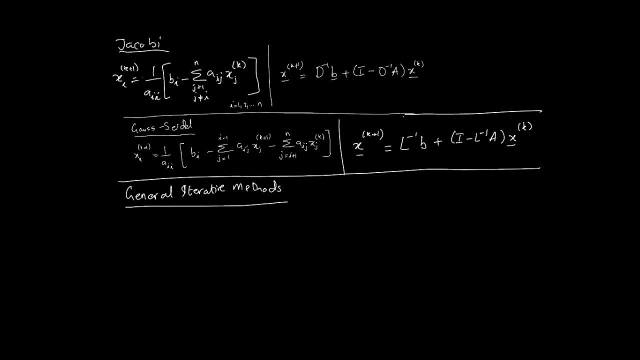 gauss idle written in matrix form. so here you see, uh, quickly summarized the jacoby method and the gauss idle method in matrix form. now what we want to do is basically look at essentially how these methods can be generalized into any general iterative method and basically that any general 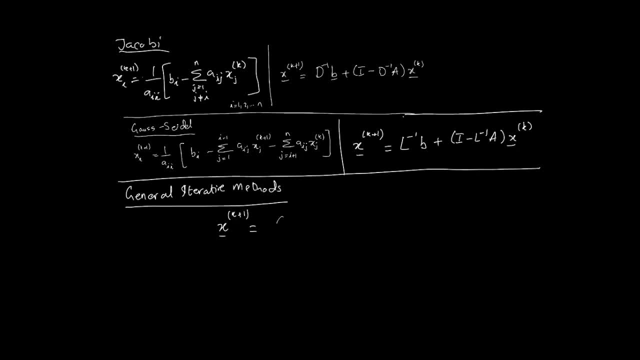 iterative method can be considered in matrix form as having some matrix g that multiplies the xk term and some matrix h that multiplies the right hand side b term, in other words. so now usually this: where the iteration, iterative iteration, matrix g, so where g is in fact i minus. 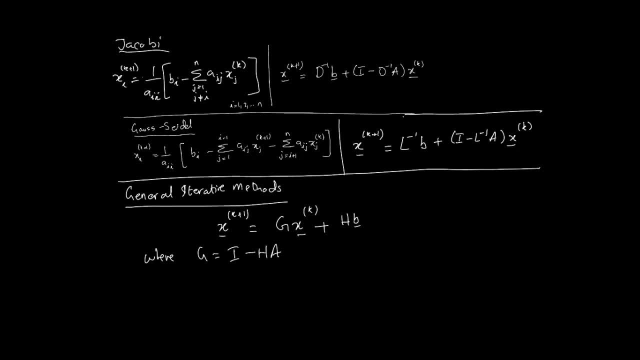 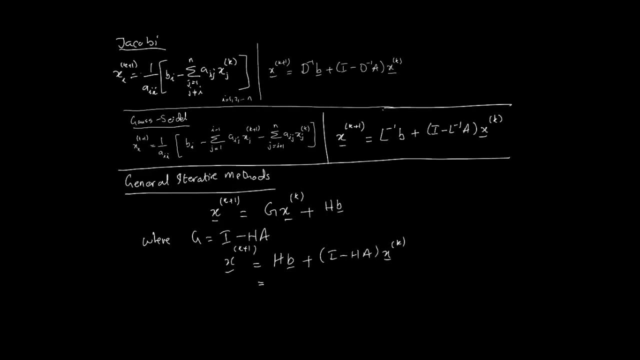 h a. okay so, and h is some approximate inverse of a, so this can be rewritten as: basically, by taking the two, the h, together, we can combine this and say that the i times xk, so these two multiply to give us just xk. okay, and plus the h b, minus h a xk. we can combine into simply saying the following: h times. 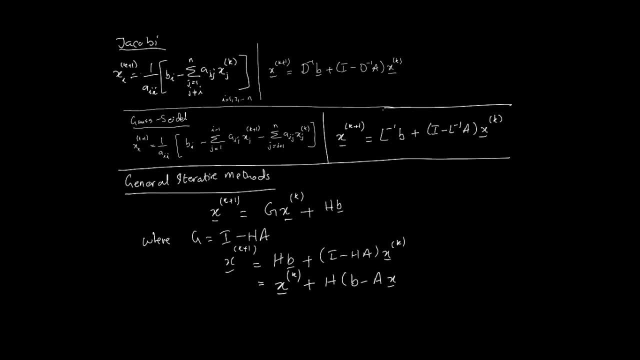 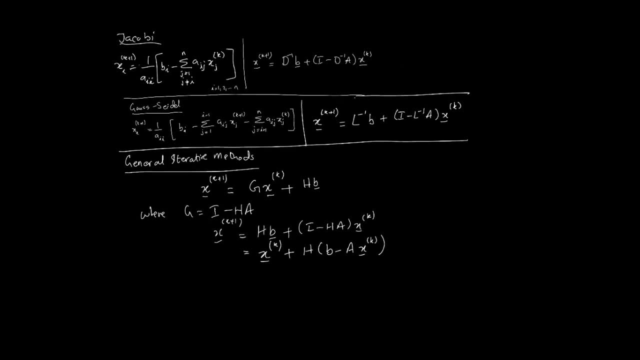 b minus a xk. okay, by just rearranging the equation now, that would mean, uh, that would finally say that we can finally say then that hey, this, this thing here, you see here, okay, this is something we've seen before- which is the residual. so essentially it boils down to just: 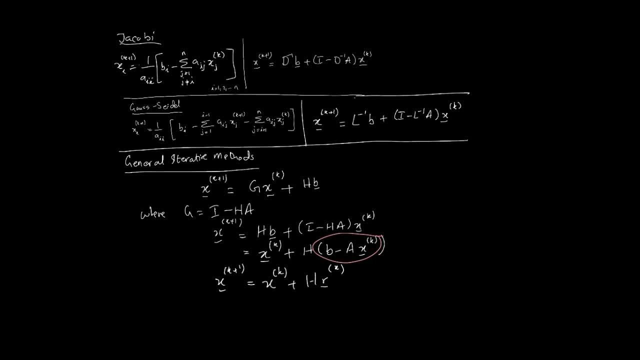 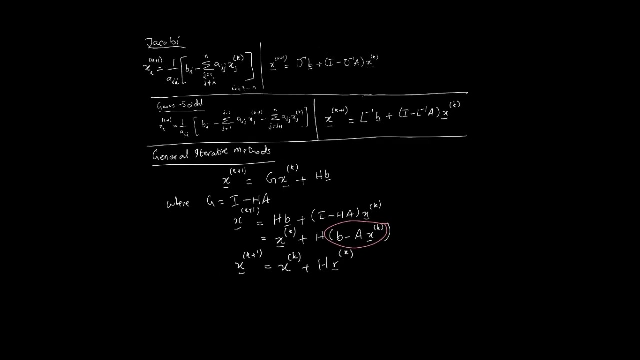 h times the residual at the kth, iterate, so um. that's just a figurative way of looking at basically what goes on um in an iterative uh method. so um, the next important thing we need to do is to connect the the iterative methods we've looked at. 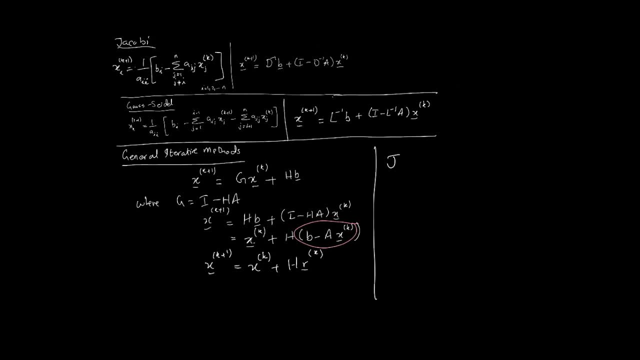 with these. so for the jacobi, so for the jacobi, if you compare, we clearly see that h is equal to d inverse. uh, okay, and and for the gaussidal? okay, for the gaussidal, h is equal to, in fact, l inverse. and now, if you look at these, um, you can clearly see that. 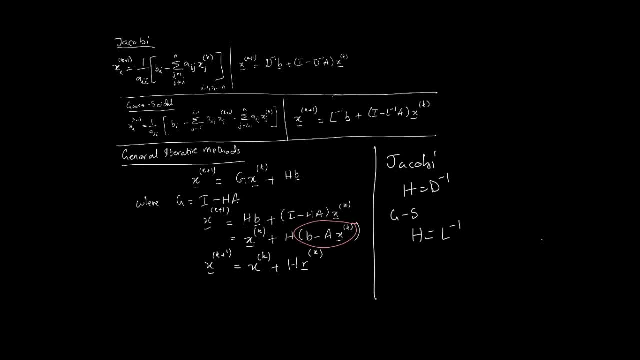 this matches very closely- not closely exactly- with these, uh, general iterative methods. uh, so that basically is in a nutshell, um how one can structure general iterative methods. so we'll stop here, thank you.